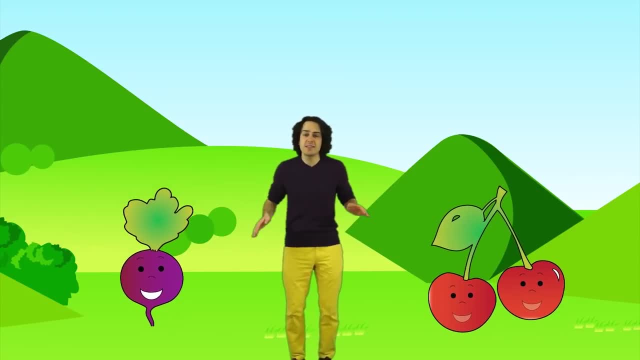 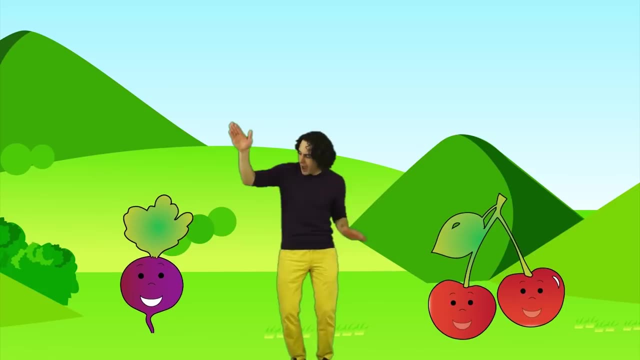 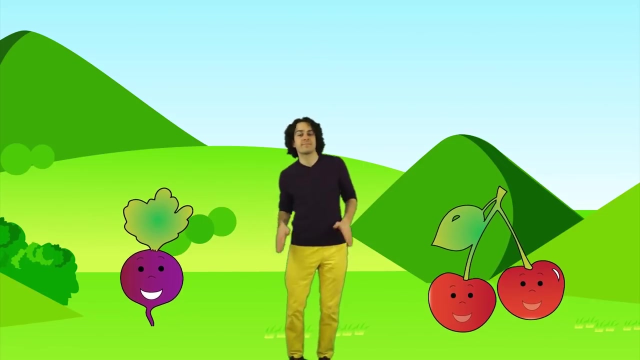 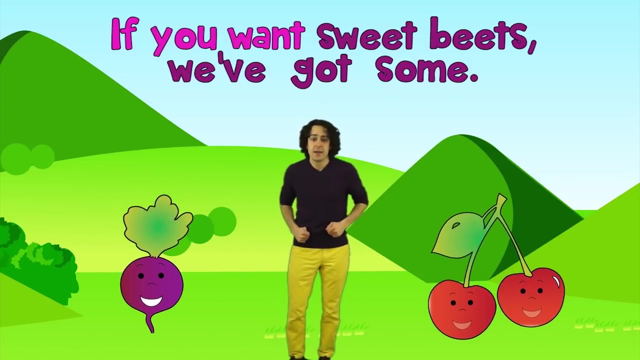 So let's tap on our legs. This is how we keep the beat nice and steady. That's it. You can play with two hands, or you can try going back and forth between your hands. So the song goes like this: If you want sweet beats, we've got some. 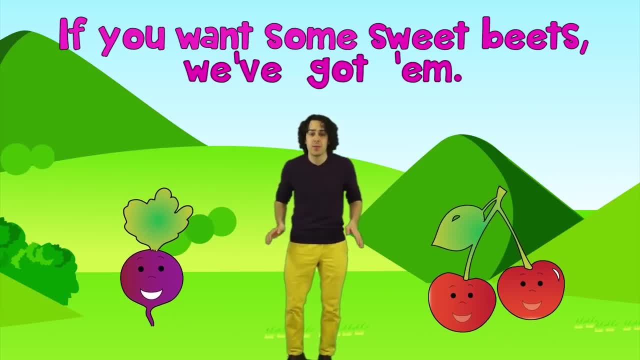 If you want some sweet beats, we've got some. If you want sweet beats, we've got some. If you want some sweet beats, we've got some. Repeat after me, Here we go, Beat beat, cherry beat. 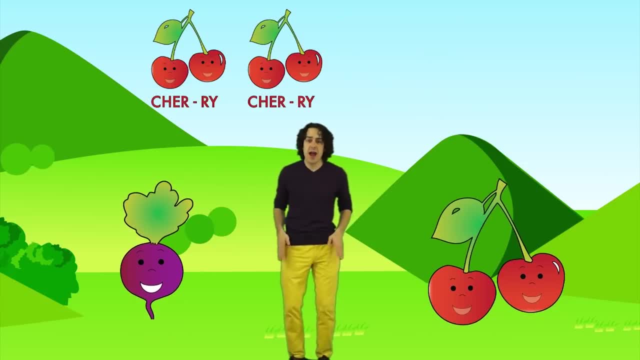 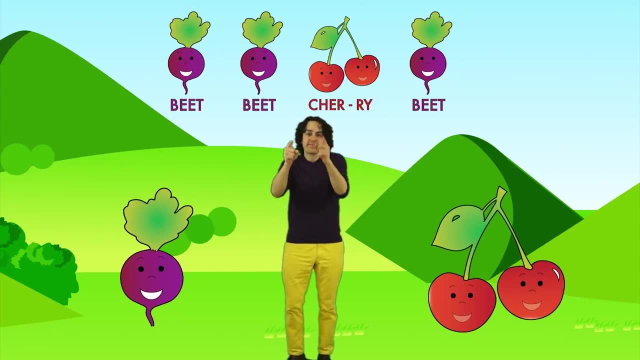 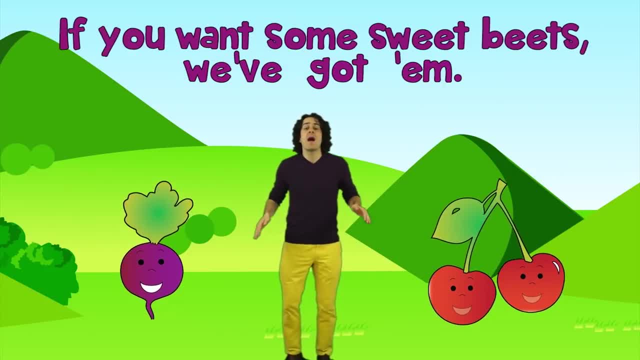 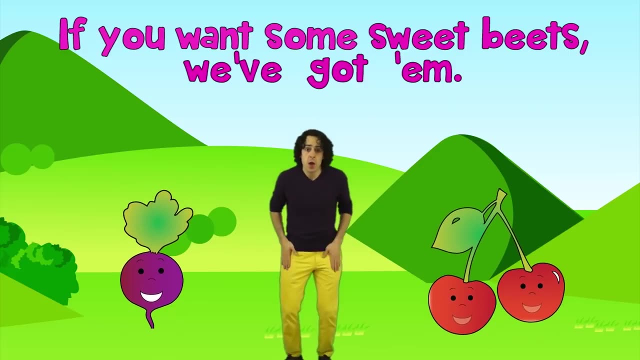 Sweet beats, we've got some. If you want some sweet beats, we've got them. If you want some sweet beats, we've got some. If you want some sweet beats, we've got them. Repeat after me again: Cherry beat, cherry beat. 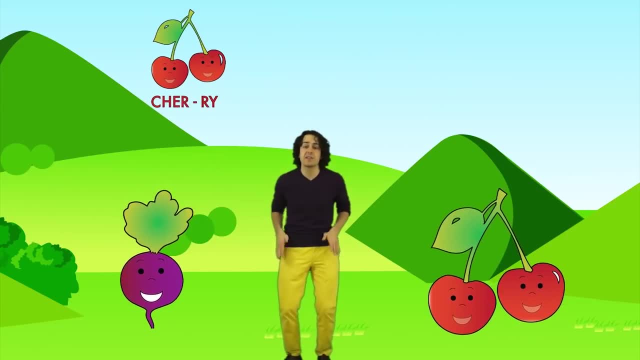 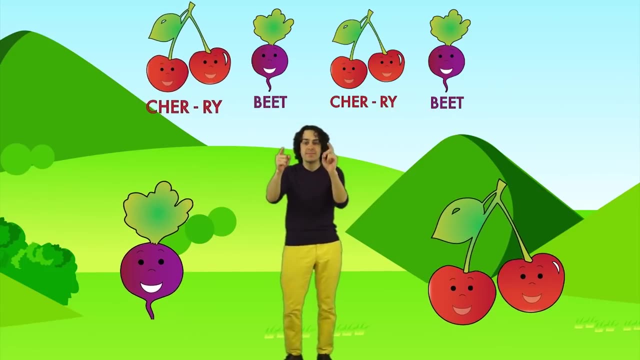 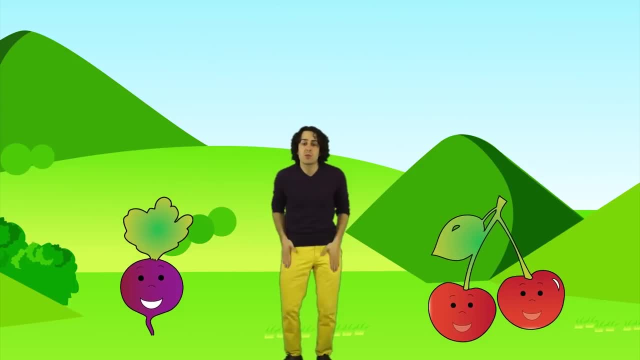 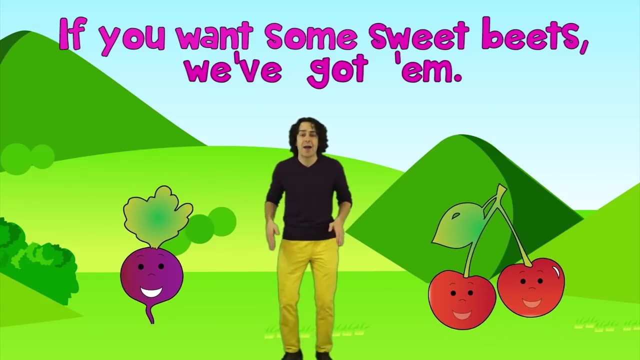 Cherry cherry cherry beat. Cherry cherry cherry beat. Sweet beats, we've got some. If you want some sweet beats, we've got them. If you want some sweet beats, we've got some. If you want some sweet beats, we've got them. 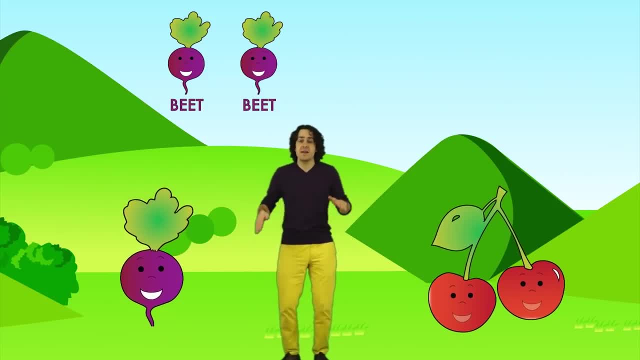 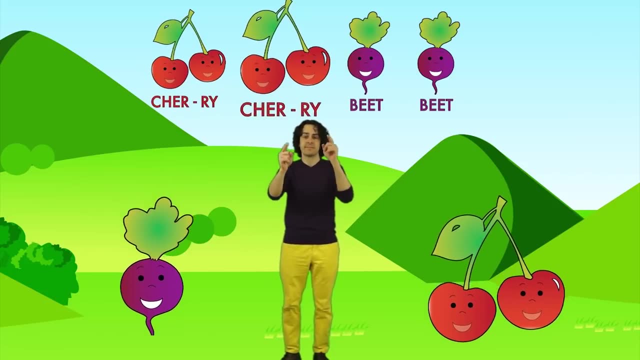 Let's put them all together. Here we go. Beat beat cherry beat. Beat beat cherry beat Cherry cherry beat beat Cherry cherry. cherry beat Cherry cherry cherry beat. 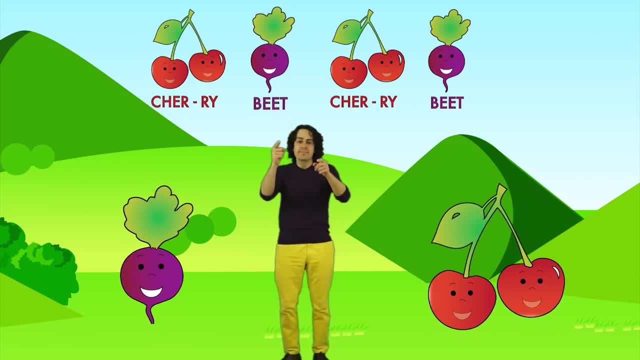 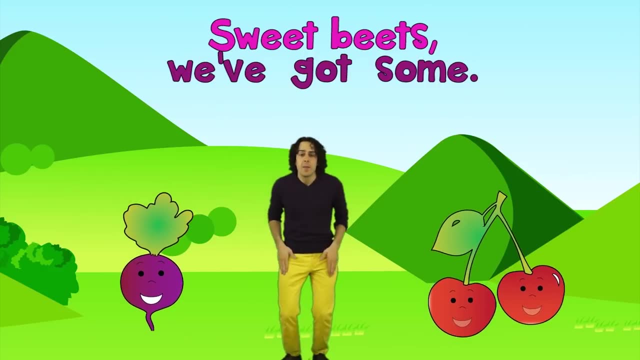